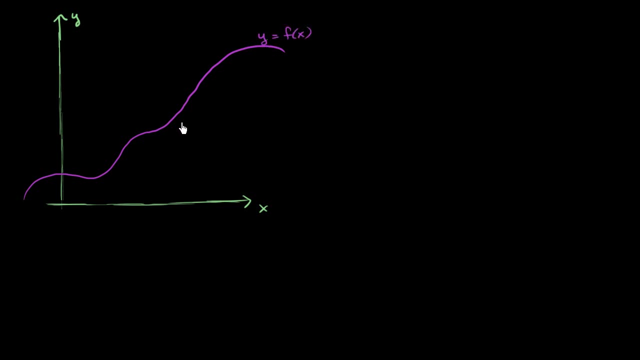 So this is the function. y is equal to f of x And just for the sake of conceptual understanding, I'm going to say it's not defined at a point. I didn't have to do this. You can find the limit as x approaches a point. 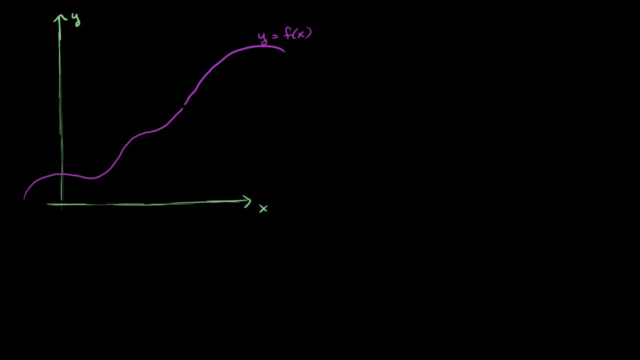 where the function actually is defined. but it becomes that much more interesting, at least for me, where you start to understand why a limit might be relevant where a function is not defined at some point. So the way I've drawn it, this function is not defined. 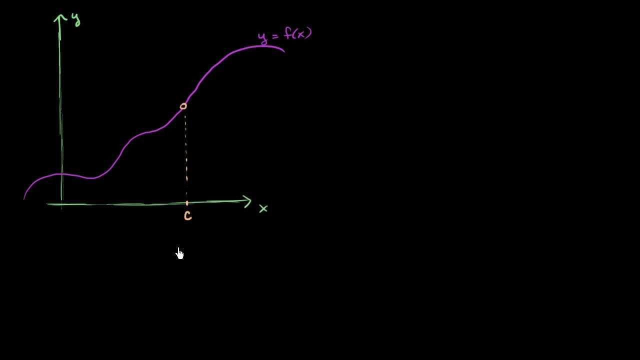 when x is equal to c. Now the way that we've thought about a limit is: what does f of x approach as x approaches c? So let's think about that a little bit. When x is a reasonable bit lower than c, f of x for our function that we just drew is right over here. 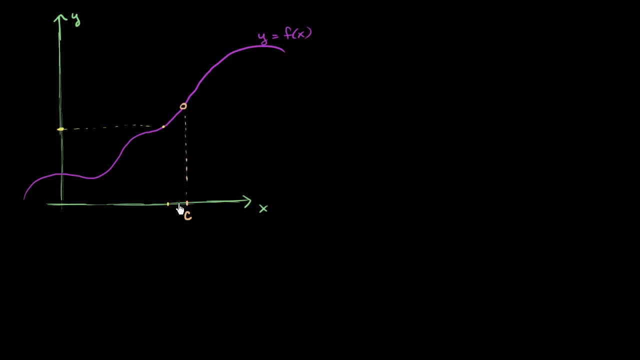 That's what f of x is going to be equal. y is equal to f of x. When x gets a little bit closer, then our f of x is right over there. When x gets even closer- maybe really almost at c, but not quite at c- then our f of x is right over here. 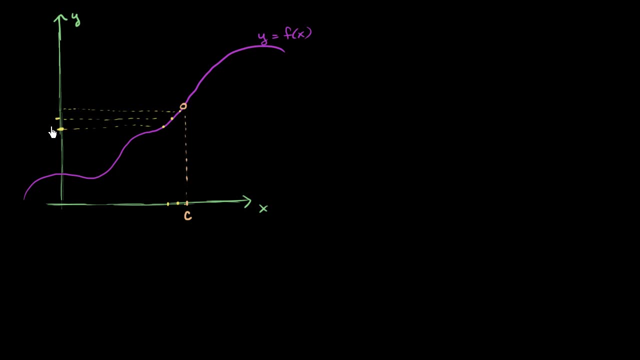 And the way we see it. we see that our f of x seems to be. as x gets closer and closer to c, it looks like our f of x is getting closer and closer to some value. It's getting closer and closer to some value right over there. 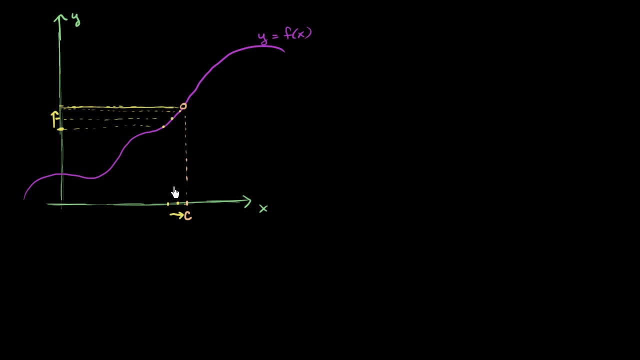 I'll even draw it. Maybe I'll draw it with a more solid line. And that was actually only the case when x was getting closer to c, from the left, from values of x less than c. But what happens as we get closer and closer to c? 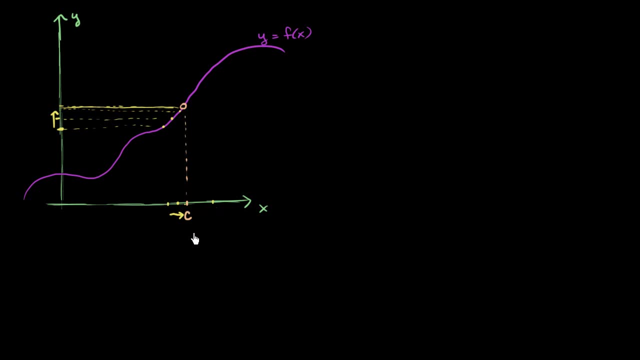 from values of x that are larger than c. Well, when x is over here, f of x is right over here, And so that's what f of x is is right over there. When x gets a little bit closer to c. 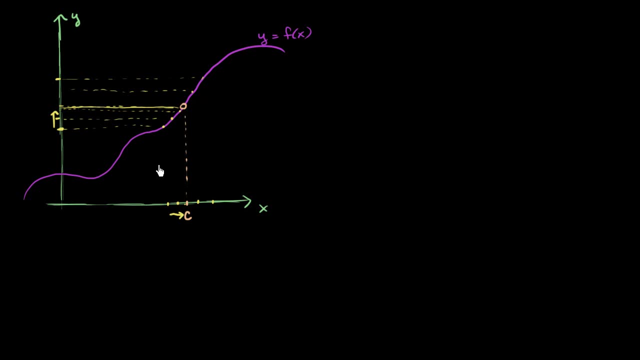 our f of x is right over there. When f of x is just very, very close to c, then our f of x is very slightly larger than c, Then our f of x is right over there. And you see, once again it seems. 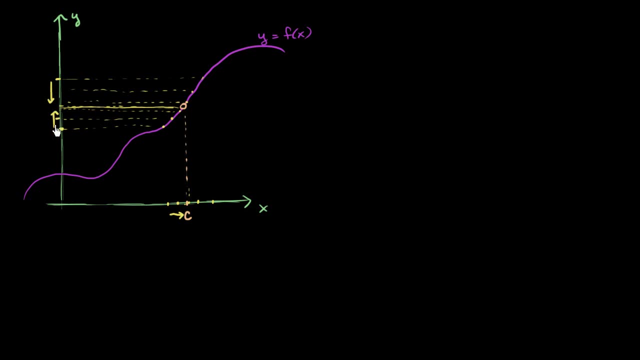 to be approaching that same value, And we call that value that value that f of x seems to be approaching as x approaches c. we call that value l or the limit, And so the way we would denote it is we would call that the limit.